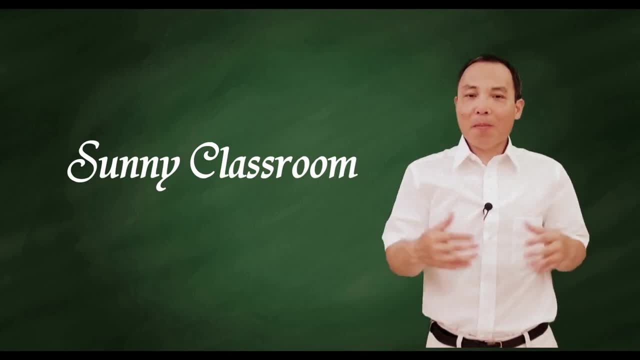 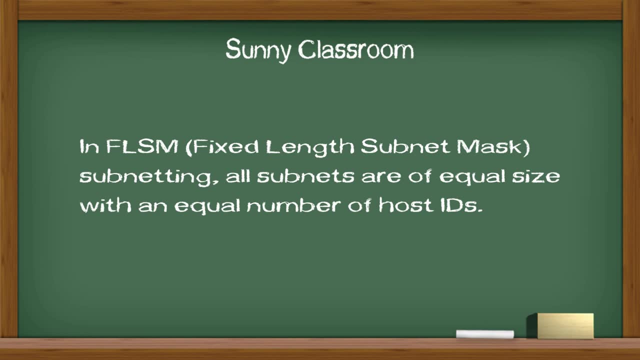 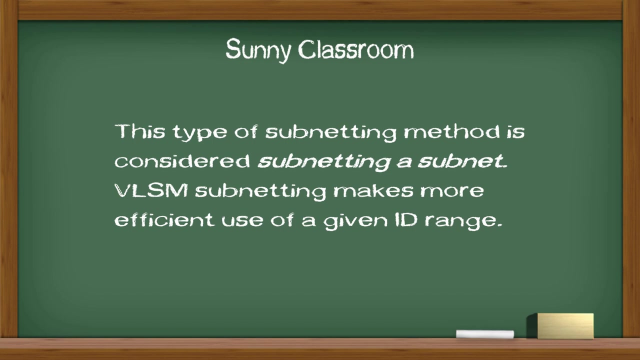 Hello, and this is Sunny. Welcome back In FLSM subnetting. all subnets are of equal size with an equal number of host IDs. In VLSM subnetting different subnets can be of different sizes. This type of subnetting method is considered subnetting a subnet. 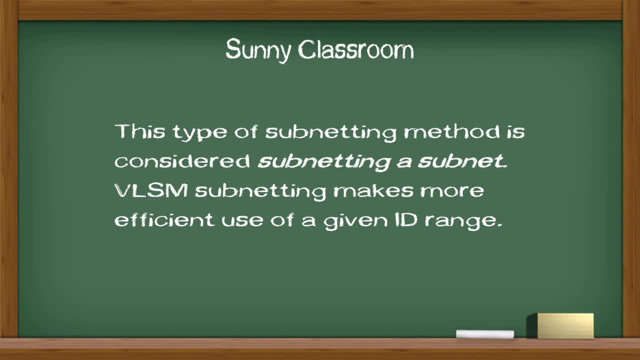 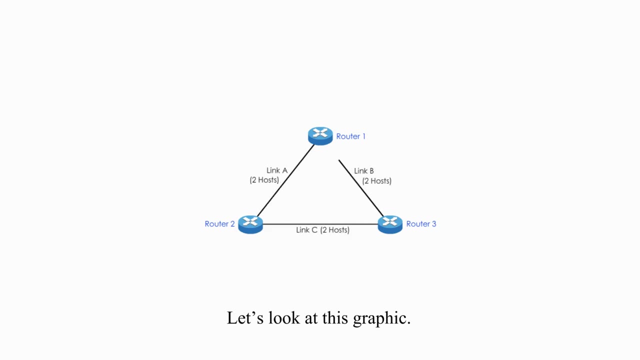 VLSM subnetting makes more efficient use of a given ID range. Today I will demonstrate in detail how VLSM subnetting works. Let's look at this graphic. Route 1 is the gateway to LAN 1 with 25 hosts. 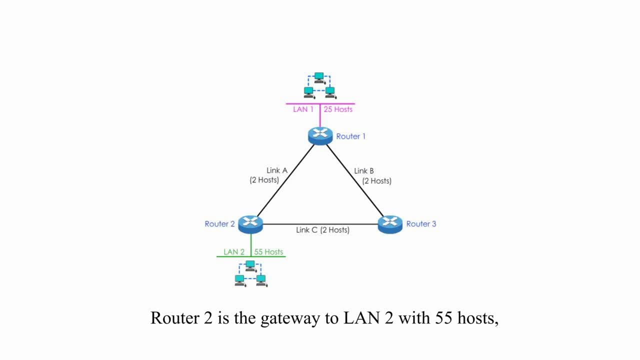 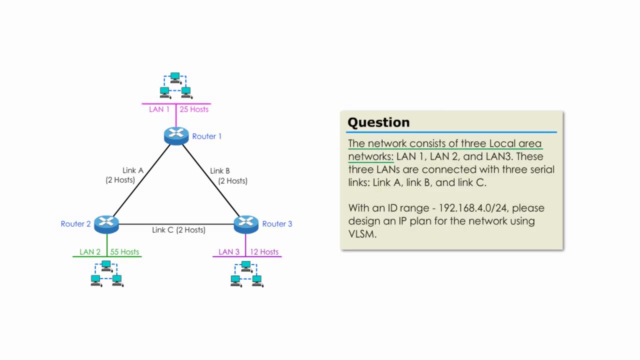 Route 2 is the gateway to LAN 2 with 55 hosts, And Route 3 is the gateway to LAN 3 with 12 hosts. Three routers are connected to each other. Here is the question. The network consists of three local area networks. 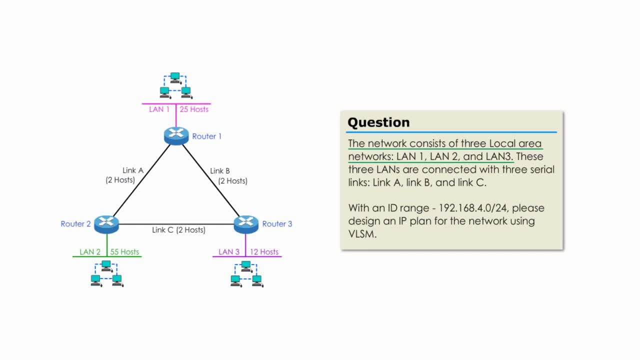 LAN 1,, LAN 2, and LAN 3.. These three lines are connected with three serial links- link A, link B and link C, With an ID range 192.168,, 4.0, 24,. please design an IP plan for the network using VLSM. 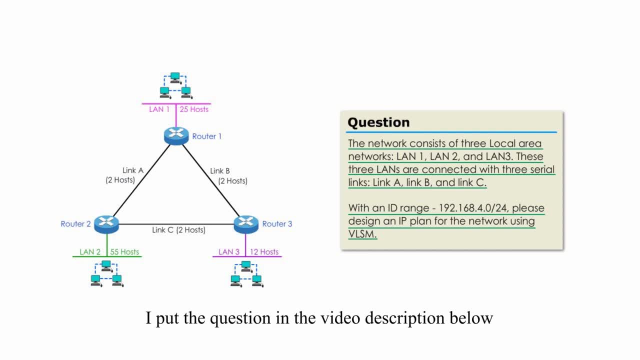 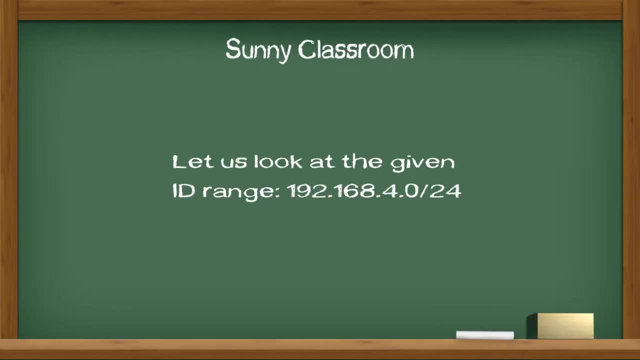 I put the question in the video description below. You can go back to the question anytime during our discussion. Let's look at the given ID range: 192.168,, 4.0, 24.. We don't care if a given ID belongs to. 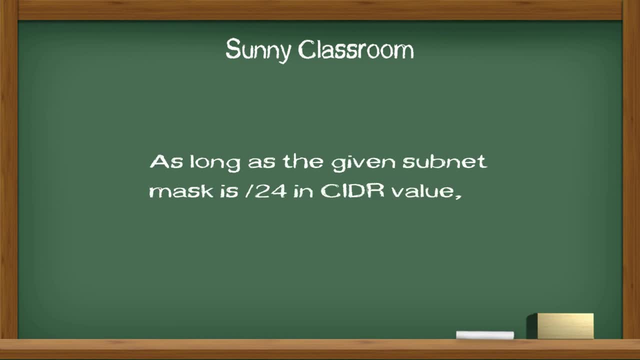 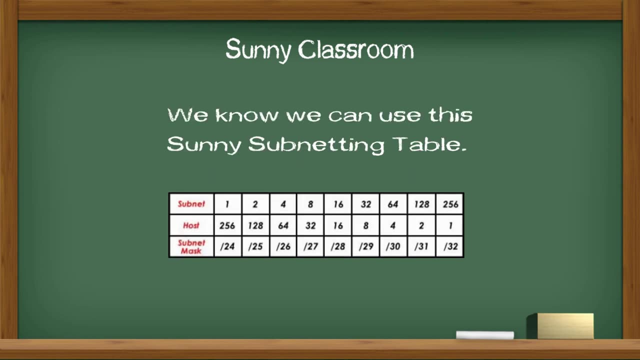 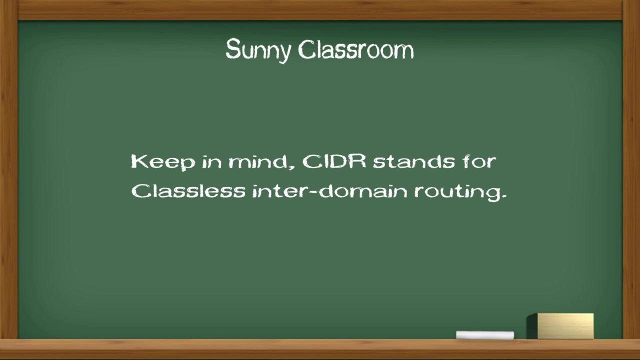 class A, B or C, As long as the given subnet mask is slash 24 in CIDR value, we know we can use this sunny subnetting table. Keep in mind CIDR stands for classless inter-domain routing CIDR. 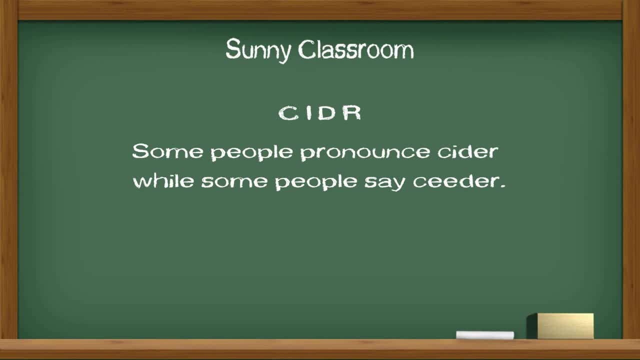 Some people pronounce of CIDR, while some people say CIDR. This reminds me a song: you like tomato, I like tomato, you say neither, I say neither. The keyword classless means forget about classes A, B or C. Whenever you see slash 24,. 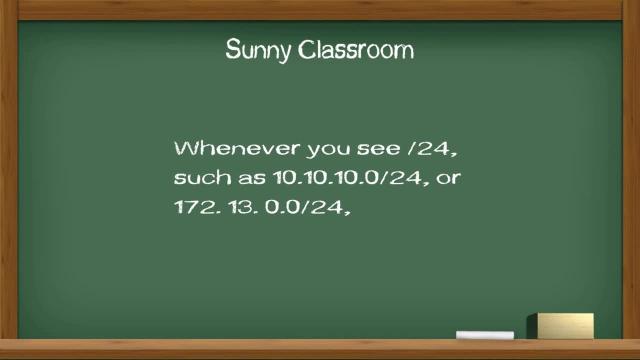 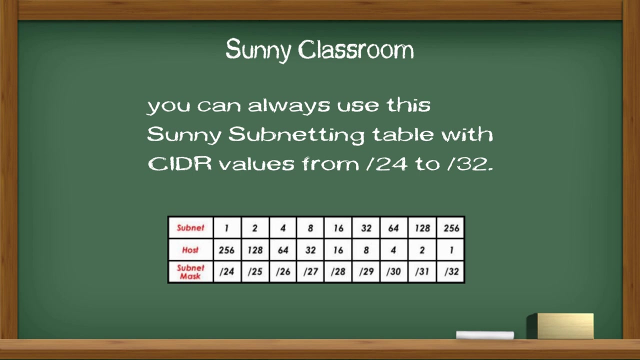 such as 10.10.10.0 slash 24, or 172.13.0.0 slash 24,. you can always use this sunny subnetting table with CIDR values from slash 24 to slash 32.. Back to the question. 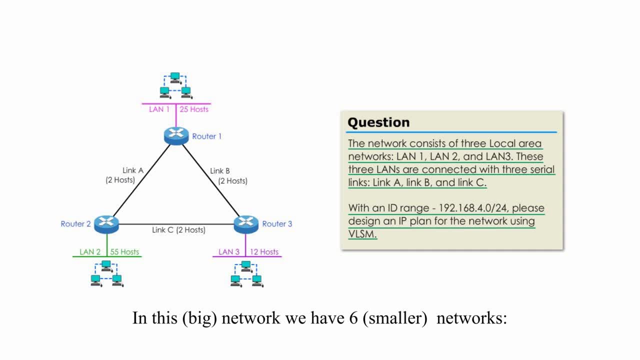 In this network we have six networks: line 1,, line 2, line 3,, link A, link B and link C. Links A, B, C are also three separate networks and each needs two host IDs. Thus, our task is to design an IP plan. 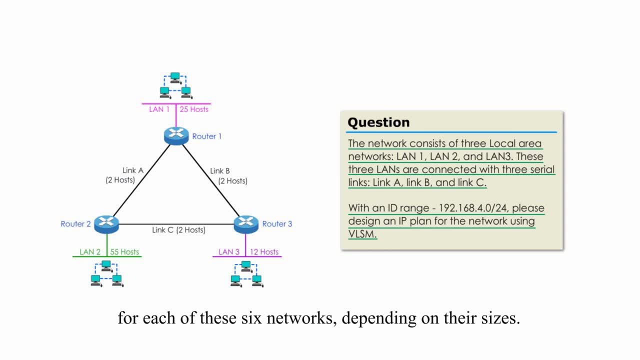 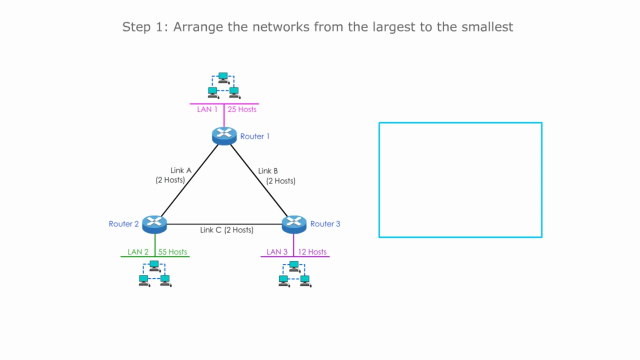 for each of these six networks, depending on their sizes. Thus, we use VLSM subnetting method. We need five steps to solve the problem. Step 1. Arrange the networks from the largest to the smallest, Thus the largest one. 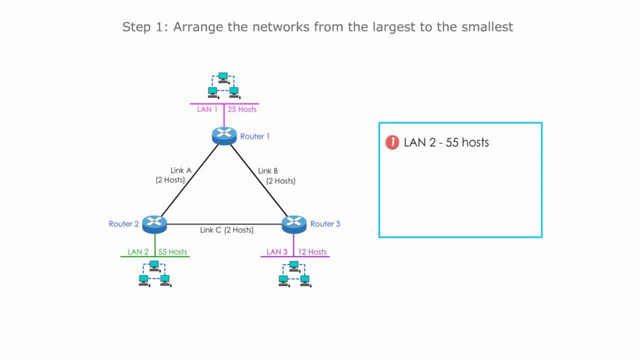 line 2 with 55 hosts. The next largest one, line 1 with 25 hosts. The third largest one, line 3 with 12 hosts, And the fourth largest one or the smallest one. links A, B and C. 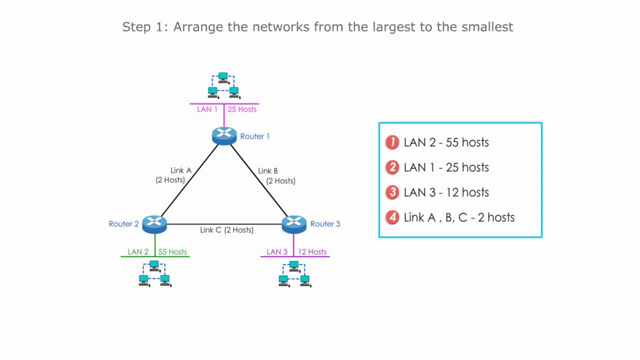 These three networks can be arranged together because they are of the same size. Each subnet needs two host IDs Once they are in a descending order. we need next four more steps to complete our task. Step 2. Pick a subnet for the largest network to use. 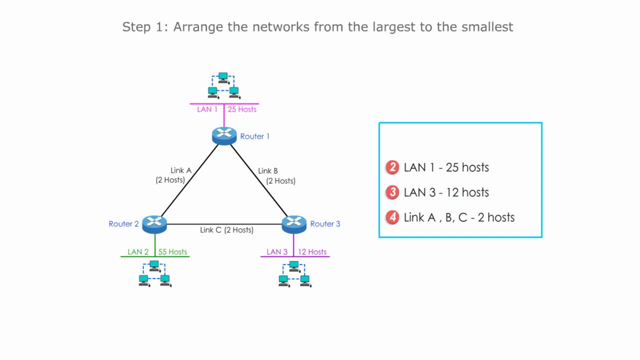 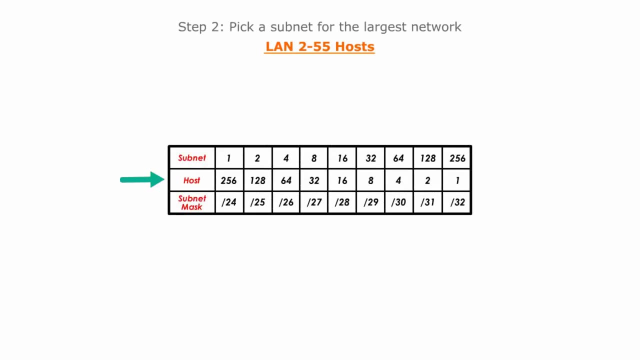 We start with line 2 with 55 hosts. Let's look at the second row in the table. We are looking for the minimum number of hosts which can satisfy line 2.. That's right, 64 is what we need. We circle 64 and the whole column. 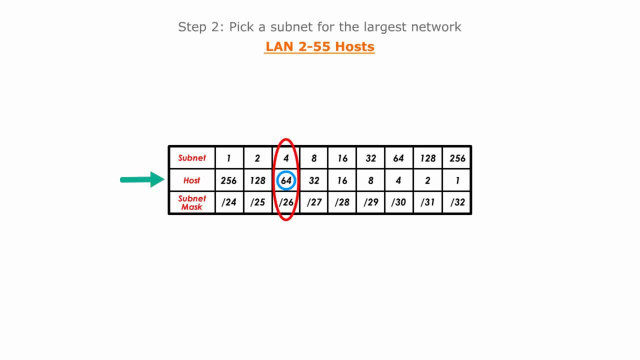 because all we need are these three numbers in this column: 4, 64, 26.. 4 means four subnets. 64 means each subnet has a total number of host IDs. 64, 26 is a new number. 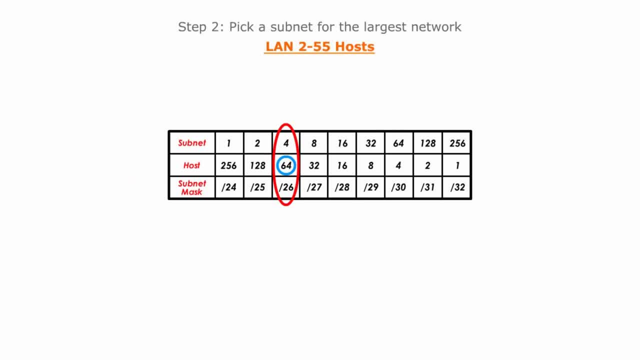 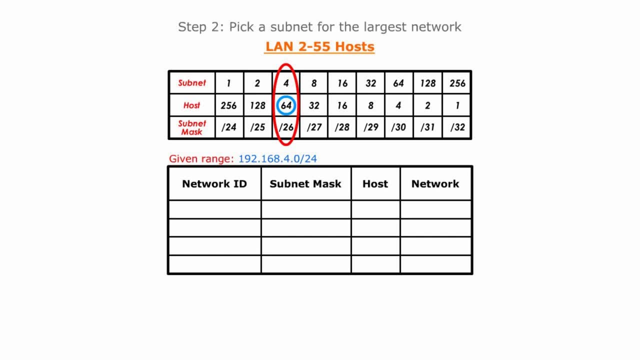 64 is the total number of host IDs. Now we will use these three numbers to build a new table with network ID, subnet mask, insider value- host- the network. Let's fill in the columns with subnets mask and host first, with slash 26 and 64. 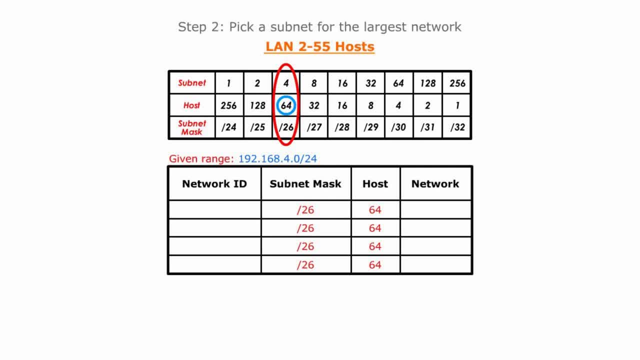 And these two numbers are directly from the column In the host. column 64 is the total number of host IDs. Keep in mind the first host ID is reserved for the network ID and the last host ID is reserved for the broadcast ID. 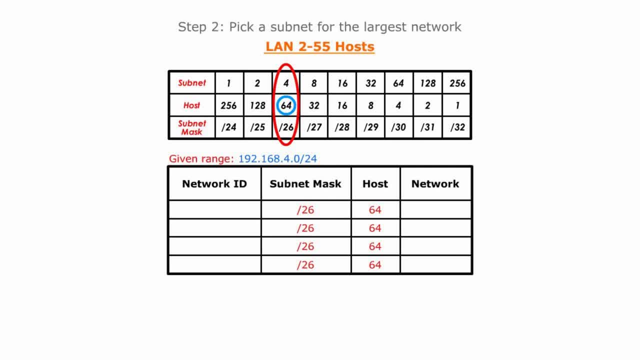 The total number of usable host IDs for each subnet is 62.. Now let's list network IDs for each subnet. The first network ID is always the original gaming ID, which is 192.168.1.. The second network ID is 192.168.4.64.. 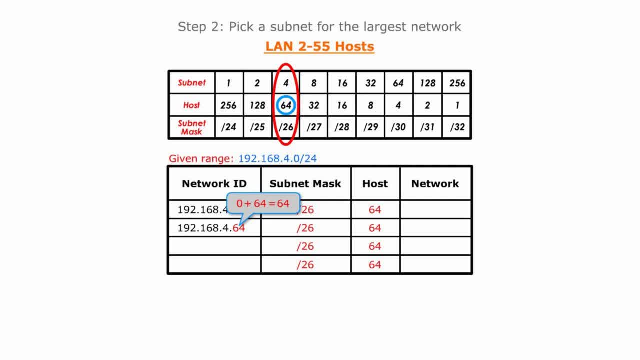 The first three octets remain the same and only the fourth octet changes. Thus we only focus on the fourth octet. The third network ID is .128.. The fourth network ID is .192.168.1.. Here is the pattern. 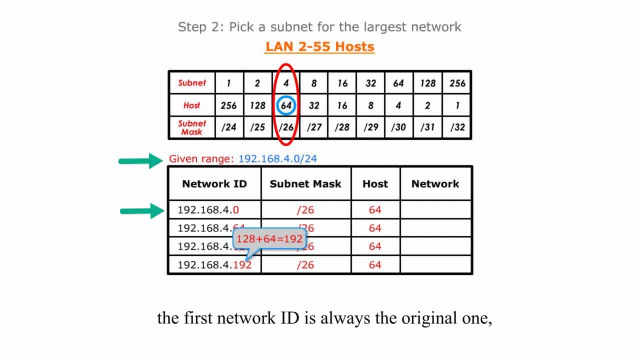 The first network ID is always the original one. The next network ID is obtained by adding 64 to its previous one. We can assign any of these four subnets to LAN2, because they are all equal size. For the sake of simplicity, we assign the first subnet to LAN2.. 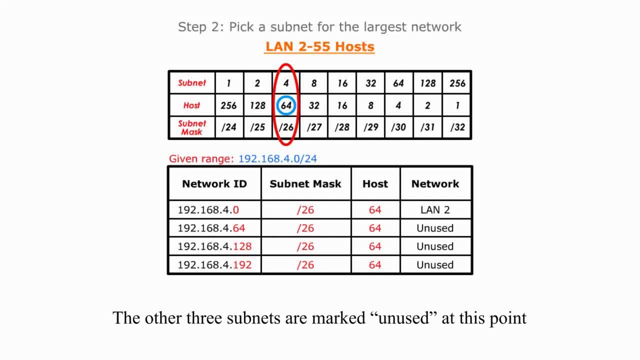 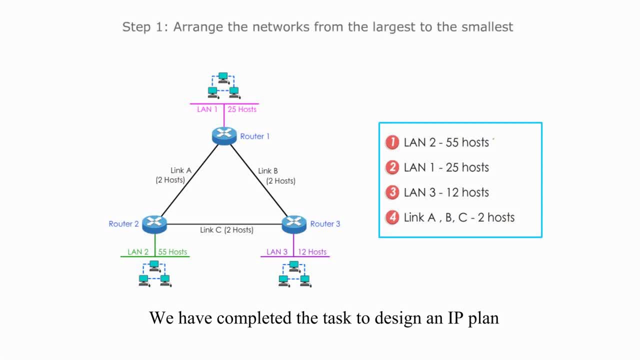 The other three subnets are marked unused at this point and they are for future use. We have completed the task to design an IP plan for the largest network, LAN2, and move to the next step: find a subnet for LAN1 with 25 hosts. 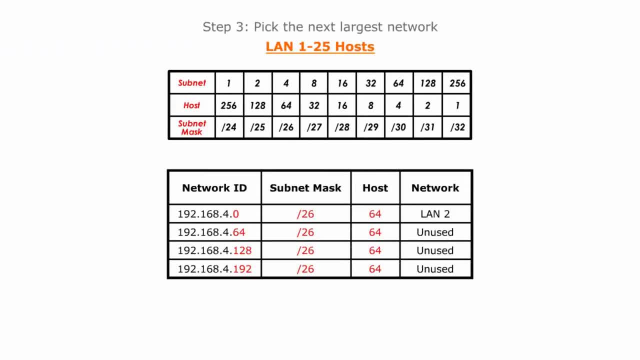 Step 3, pick the next largest network to work with. Step 3 repeats the process of step 2.. First look at the second row in the SONY table. We are looking for the minimum number of hosts which can satisfy LAN1 with 25 hosts. 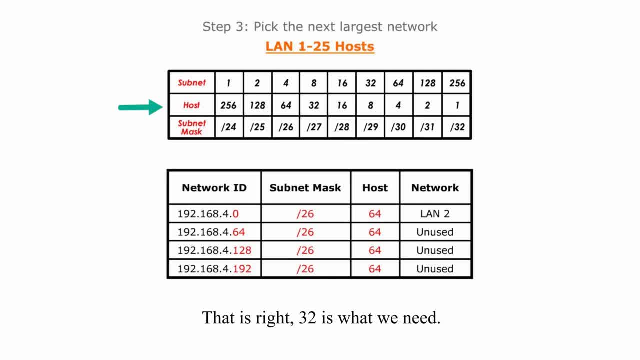 That's right. 32 is what we need. We circle 32 and the whole column, because all we need is this column. Let's look at the second table. We select the first unused subnet and subdivide it into two smaller subnets. 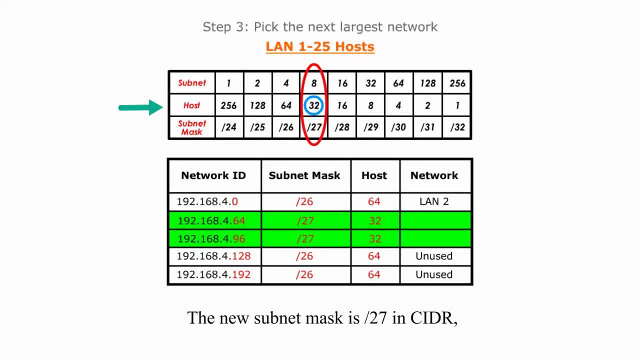 The new subnet mask is select27,- Insider, and the total number of host IDs is 32, which can satisfy LAN1, which only needs 25 host IDs. Dividing one subnet into smaller subnets is called subnetting a subnet. Let's choose 192.168.4.64.27 for LAN1. 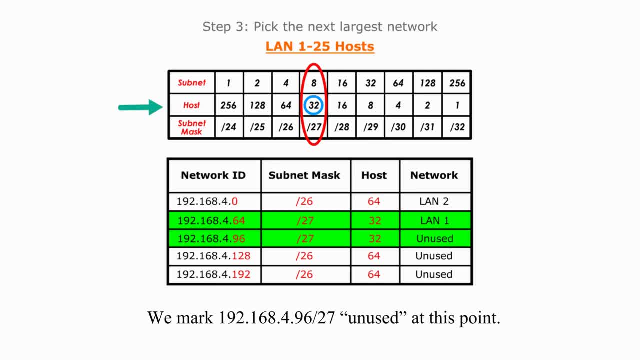 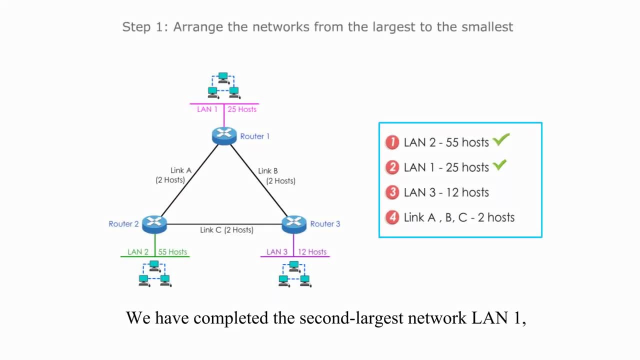 And we mark the second one, 192.168.4.96.27, all used at this point, reserved for the future use. We have completed the second largest network, LAN1., And we move to the next step: find the subnet for LAN3 with 12 hosts. 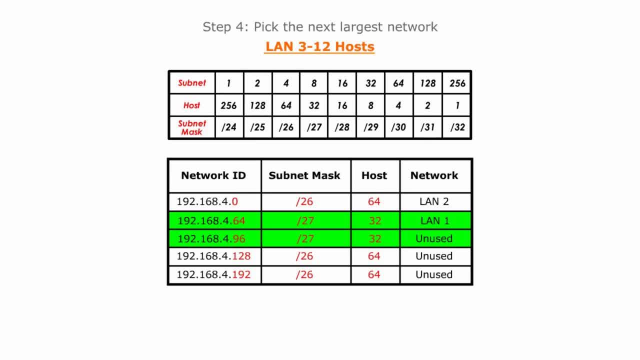 This step repeats the process above. Let's look at the second row in the sunny table. We are looking for the minimum number of hosts which can satisfy LAN3 with 12 hosts, 16 is the number We circle, 16 and the whole column. 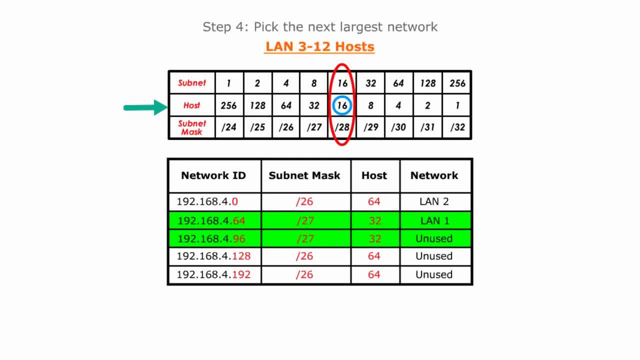 Now we want to subnet the all used network 192.168.4.96.27 and further divide it into two smaller subnets. With the new subnets mask slash 28 with 16 total host IDs, We choose 192.168.4.96, slash 28 for LAN3. 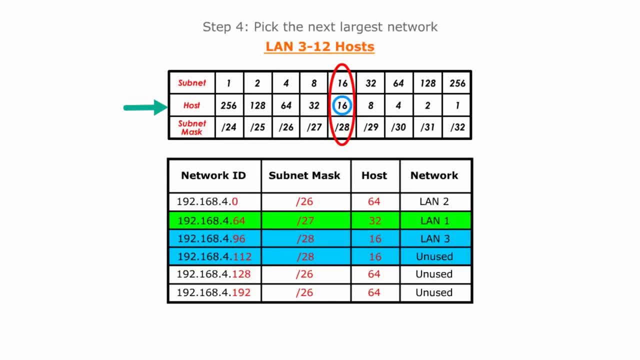 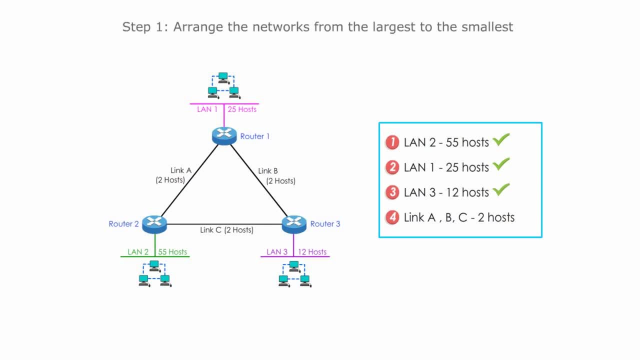 And we mark 192.168.4.112, slash 28,, all used at this point and reserved for the future use. We have completed step four and we move to the last step. We want to assign three smaller subnets for serial links: A, B and C. 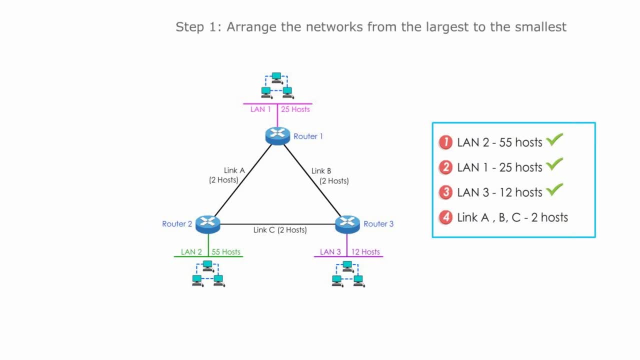 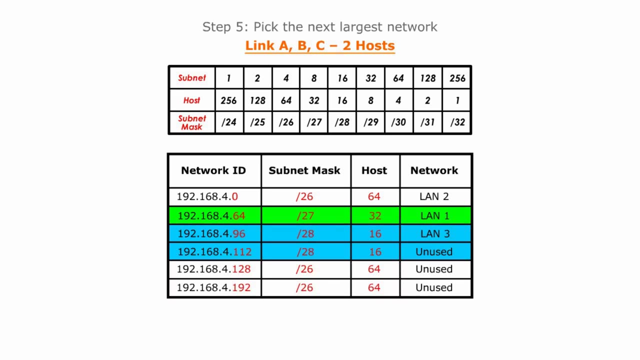 Each link needs two host IDs. Step five is the last step, because once we get subnets for these three links, we are done. Let's look at the second row in the table. We are looking for the minimum number of hosts that can satisfy a network with only two hosts. 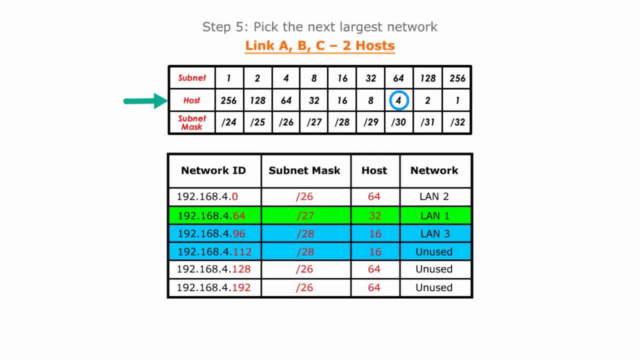 We believe the number four is what we are looking for. We circle four and the whole column. We can see the new subnet mask is slash 30. We choose the all used subnet, 192.168.4.112, slash 28, to further divide it into four smaller subnets. 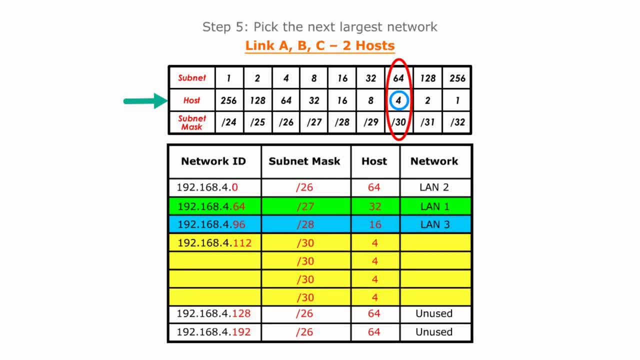 Why four smaller subnets? I leave this question to you. Now let's fill out these four new rows. We only focus on the fourth octet Instead of reading the whole IP addresses. I believe you are already tired of my accent. The first one is dot 112, slash 30.. 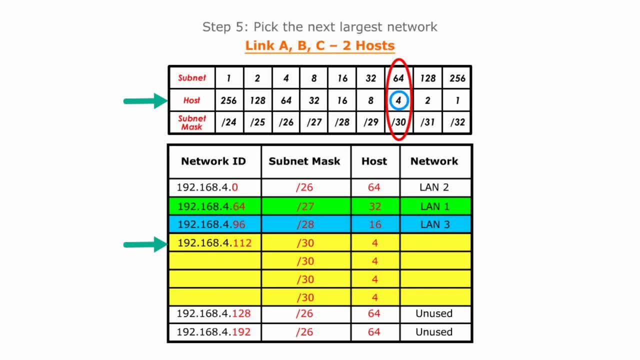 The second one is dot 116 slash 30.. The third one is 120 slash 30.. The fourth one is 124 slash 30.. Each subnet has four host IDs, which are exactly what we need. The first ID is reserved for the network ID. 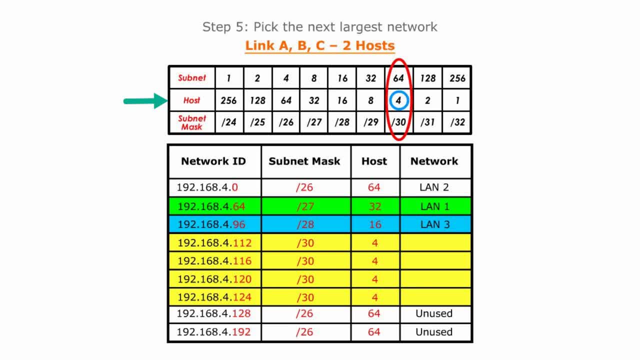 The last one is reserved for the network ID, The last one is reserved for the broadcast ID And two useful IDs are assigned to two routers on each link. We can assign any three out of four subnets to links A, B and C.